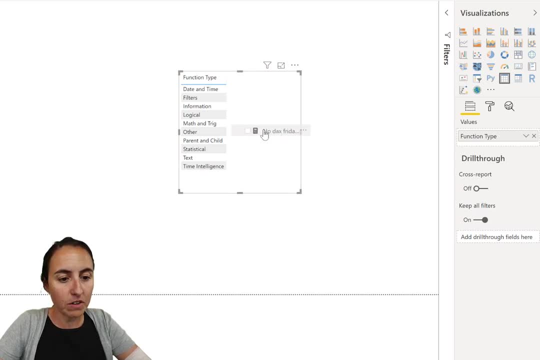 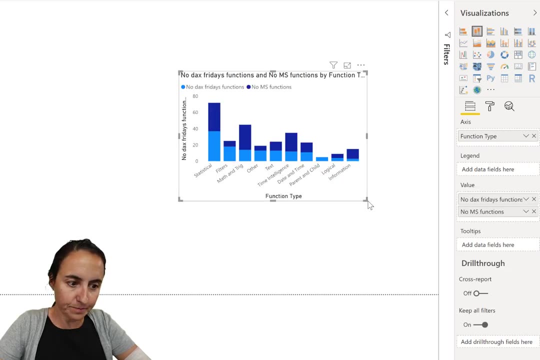 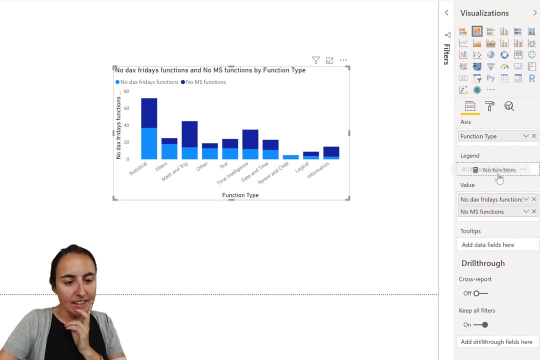 have the function type, and then we need to have the number of DAX Fridays, and the number of this is a bad name. it should be called like functions left to do for DAX Fridays, because it is what it is. So now, if I add the total, 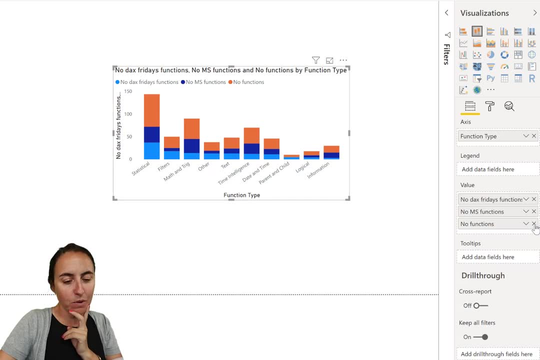 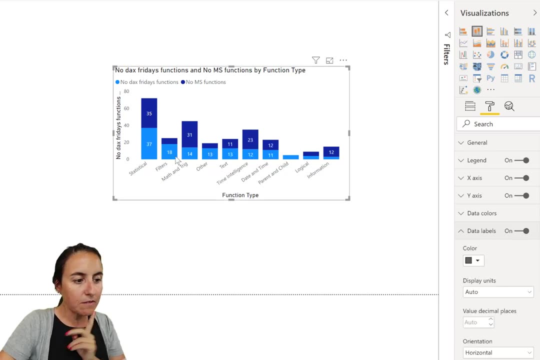 which is in there. you know we'll add it on top. That's not what we want. So if I put here the add data labels, it will give me the labels for each individual part, but it will not give me. there's no way to say show total, which it should be, but there's not. So how do you do it? Okay, 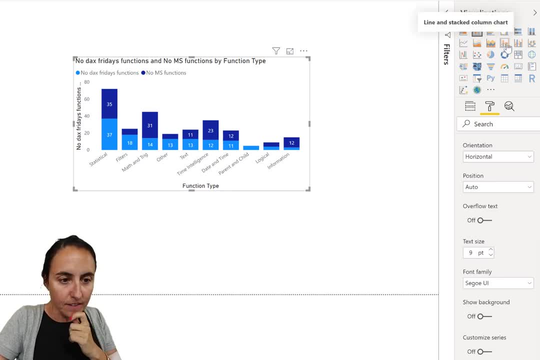 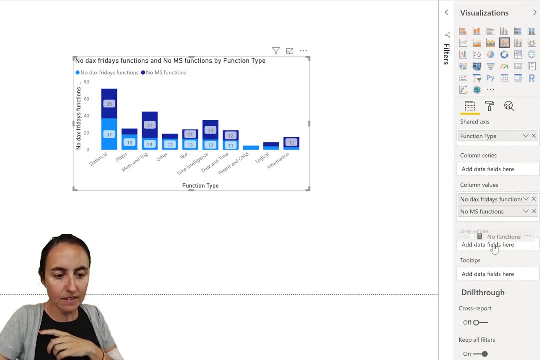 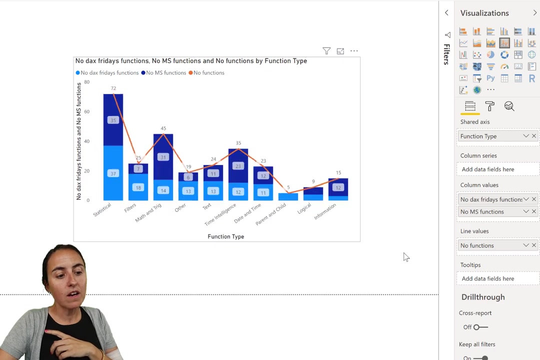 let's do it. We're going to convert this into a stacked column chart and line, okay, And we're going to add as a line the total value. So this is the total And you can see here that it starts to appear. but obviously we do not want to have a line chart that. it would make no sense, You can. 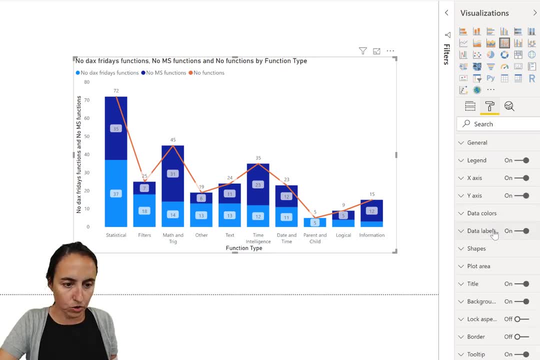 turn that off If you go to to, to, to, to. I always forget how to do this. Um, shapes, stroke, Okay. So with these you say to Power BI: chart how thick you want the line to be And in: 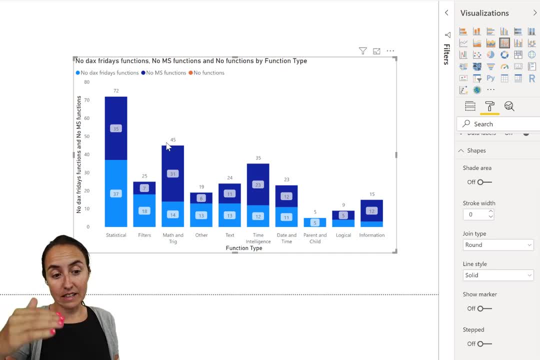 this case, we want no line, So we have to have the stroke of the line zero and then it disappears. And I recommend you to do another thing, and is to go to data labels and then customize series And then for the totals, which is the number of functions. 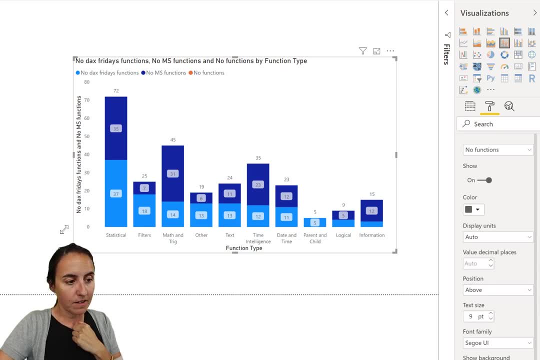 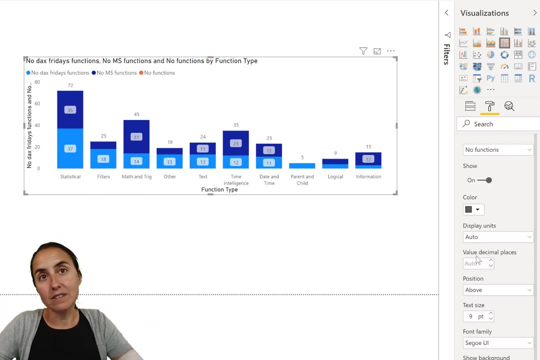 put the position always above. Okay, So you always, otherwise it will just start moving around and you always want that one above. Let the other ones order, because otherwise you're going to have a mess. But now you can see that there are 72 functions. I've covered 37 for statistical. 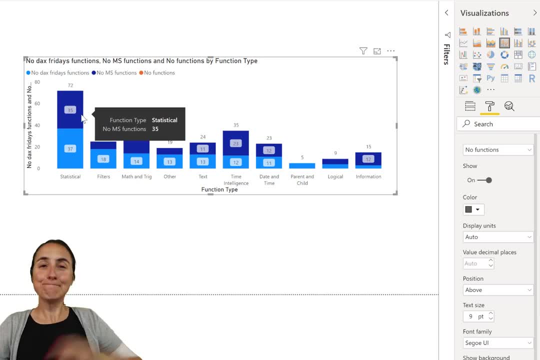 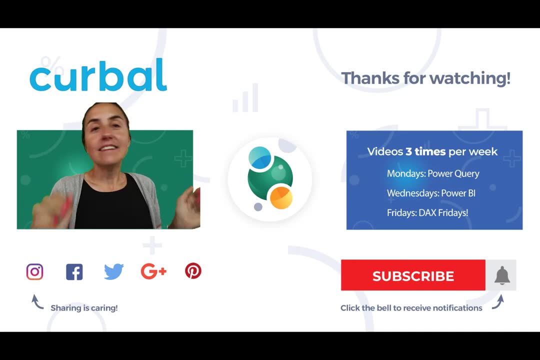 functions. I have 35 left to do. Cool, right, Awesome trick. Thank you, Reza, for sharing that with us, And that's all for today. So I will see you again on Friday with another DAX- Fridays Until then. 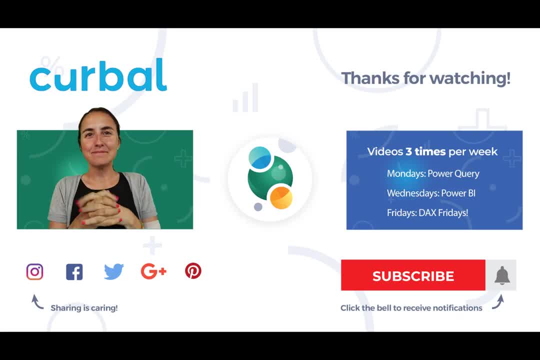 take care and bye, bye.